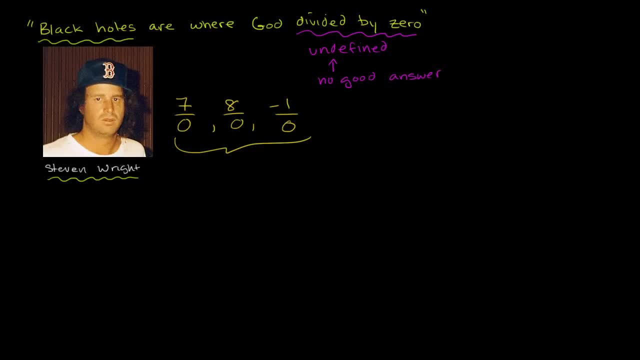 And we could just take the simplest of all non-zero numbers. we'll just do it with one, but we could have done this with any non-zero number. Let's take the example of black holes. We have one, and since we don't know what it means, 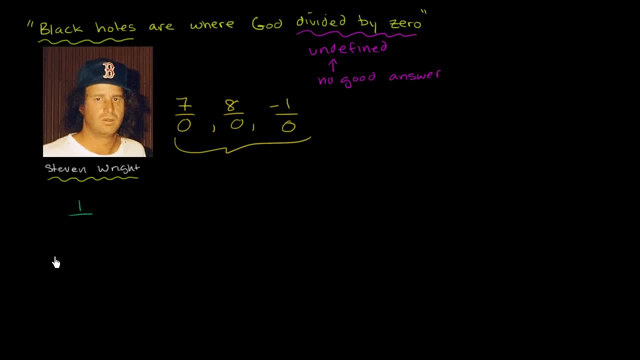 or we're trying to figure out what it means to divide by zero. let's just try out really, really really small positive numbers. Let's divide by really really small positive numbers and see what happens as we get close to zero. 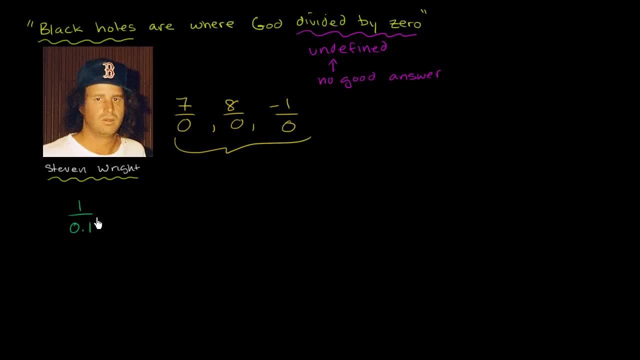 So let's divide by zero point one. Well, this will get us to ten. If we divide one by zero point zero one, that gets us to one hundred. If I let me go really, really close to zero, If I divide one by zero point zero, zero, zero, zero, zero one. 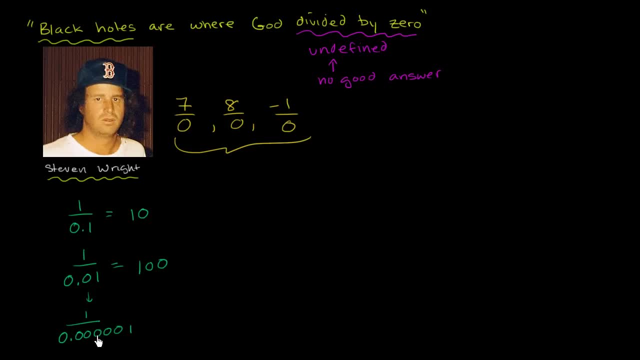 this gets us. so this is not a tenth hundredth thousandth, ten thousandth hundred thousandth. this is a millionth One divided by a millionth, that's going to give us one million. So we see a pattern here. 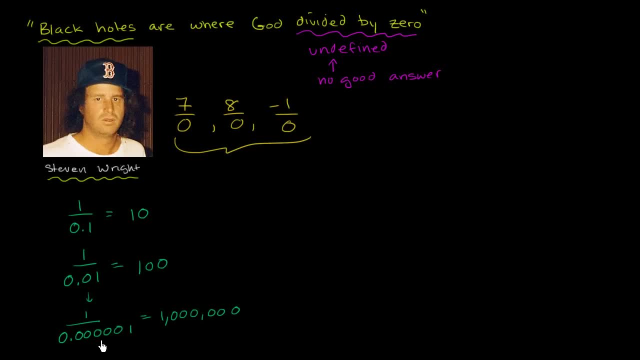 As we divide one by smaller and smaller and smaller positive numbers, we get a larger and larger and larger value. So based on just this, you might say: well, that's somewhat of a definition for one divided by zero. Maybe we can say that one divided by zero is positive infinity. 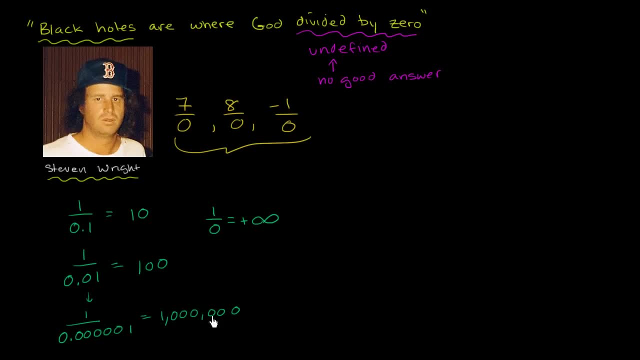 If we put smaller and smaller positive numbers here, we get super, super, super large numbers right over here. But then your friend might say: well, that worked when we divided by positive numbers close to zero. but what happens when we divide by negative numbers close to zero? 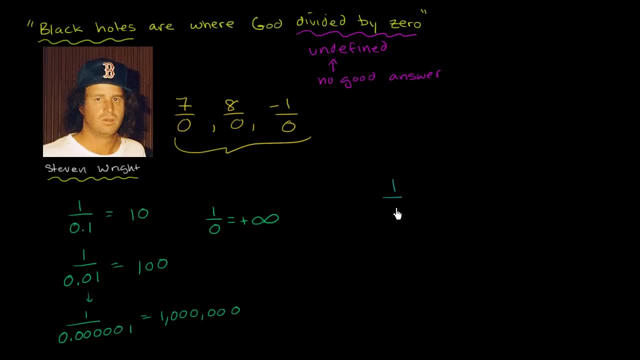 So let's try those out. Well, one divided by zero point one, or I should say negative zero, zero point one that's going to be negative ten. One divided by negative zero point zero, one that's going to be negative one hundred. 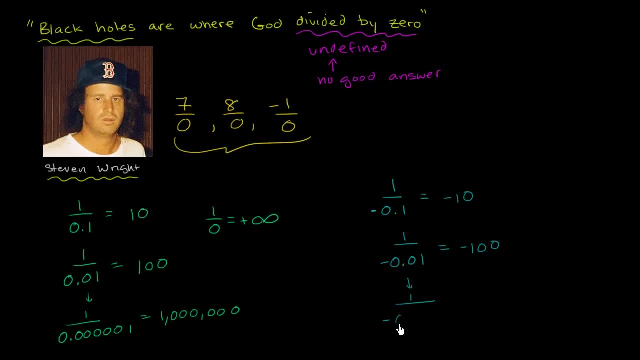 And if we go all the way to one divided by negative zero, point, zero, zero, zero, zero, zero, one, yep, I drew the same number of zeros that gets us to negative one million. And so when we see, when we keep dividing one by negative numbers,